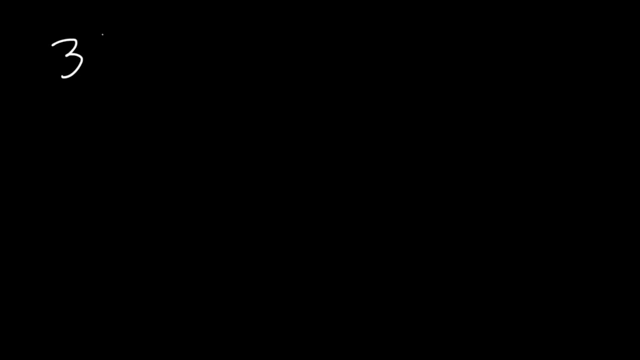 Consider the following exponential equation: 3 raised to the x plus 2 is equal to 9 raised to the 2x minus 3.. How can we find the value of x without using logs? What you need to do is change base 9 into base 3.. 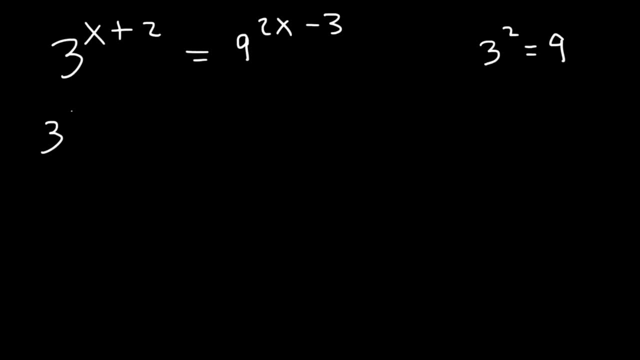 3 squared is equal to 9, so we can replace 9 with 3 squared, And whenever you raise one exponent to another exponent you need to multiply. So we've got to multiply 2 by 2x minus 3.. 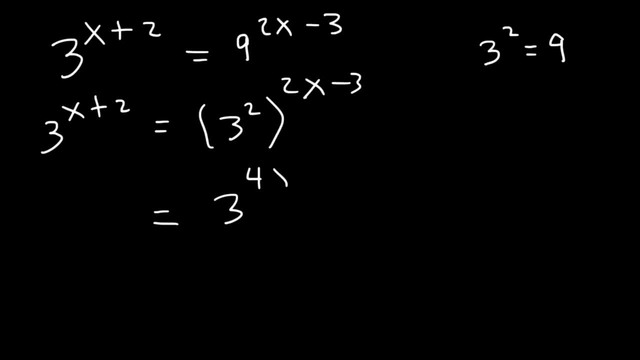 So on the right side this is going to be 3 raised to the 4x minus 6.. Now, if the bases are the same, then the exponents must be equal to each other. Therefore, x plus 2 is equal to 4x. 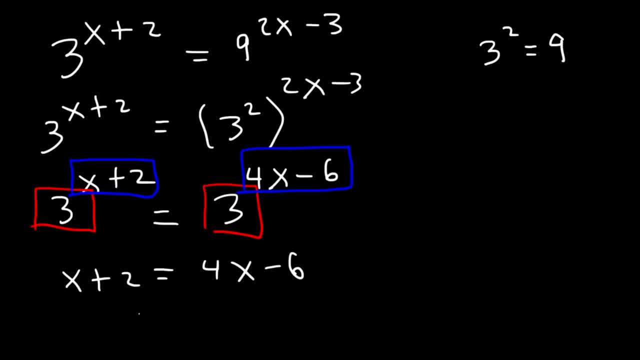 Now let's subtract both sides by x and let's add 6 to both sides, So these two will cancel. 2 plus 6 is 8.. 4x minus x is 3x, So we can see that x is equal to 8 over 3.. 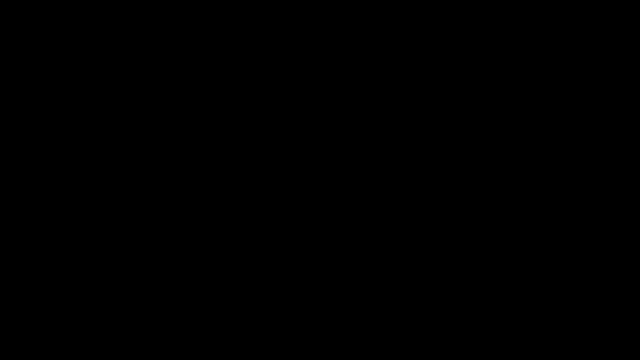 And so that's the answer for this one. Now let's work on another example. Let's work on another example: 8 raised to the 4x minus 12 is equal to 16 raised to the 5x minus 3.. 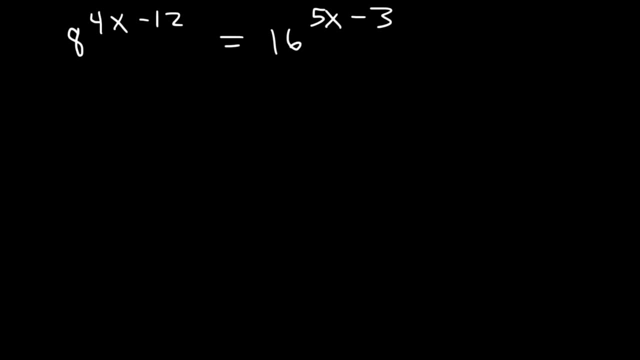 So go ahead and find the value of x. Now what we need to do is convert 8 and 16 into a common base. 2 is a multiple of 8 and 16, so 2 is the common base. 2 to the third power is 8.. 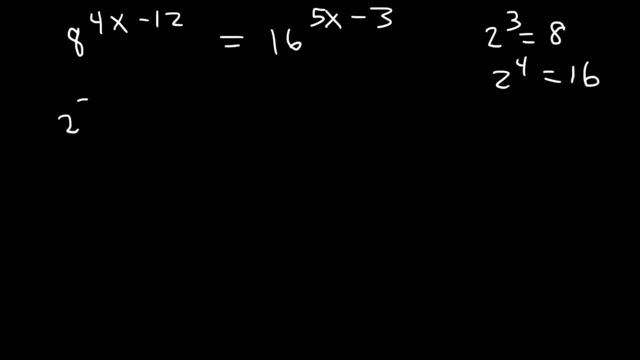 2 to the fourth power is 16.. So let's replace 8 with 2.. 2 to the third power And let's replace 16 with 2 to the fourth power. Now we need to multiply 4x minus 12 by 3.. 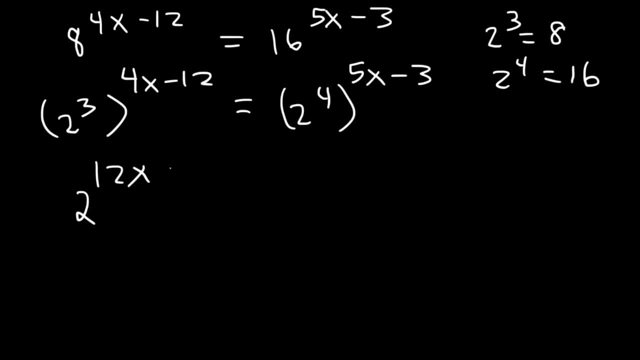 4x times 3 is 12x. 3 times negative. 12 is negative 36.. Now we need to multiply 5x minus 3 by 4. So that's going to give us 20x minus 12.. 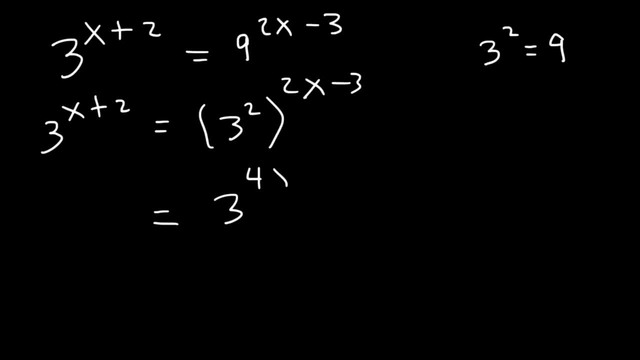 So on the right side this is going to be 3 raised to the 4x minus 6.. Now, if the bases are the same, then the exponents must be equal to each other. Therefore, x plus 2 is equal to 4x. 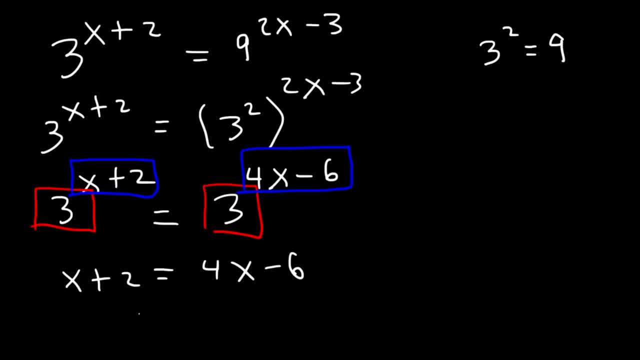 Now let's subtract both sides by x and let's add 6 to both sides, So these two will cancel. 2 plus 6 is 8.. 4x minus x is 3x, So we can see that x is equal to 8 over 3.. 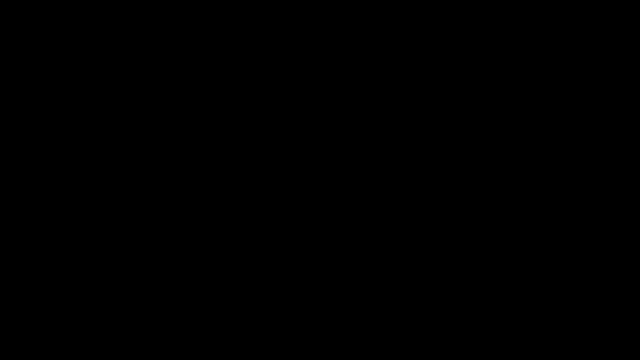 And so that's the answer for this one. Now let's work on another example. Let's work on another example: 8 raised to the 4x minus 12 is equal to 16 raised to the 5x minus 3.. 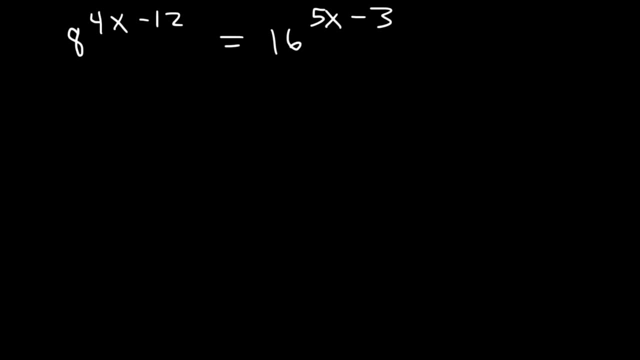 So go ahead and find the value of x. Now what we need to do is convert 8 and 16 into a common base. 2 is a multiple of 8 and 16, so 2 is the common base. 2 to the third power is 8.. 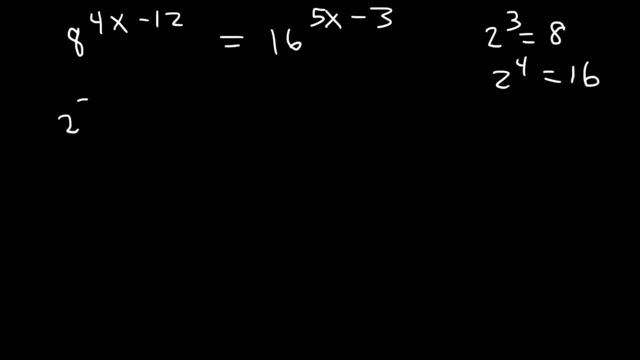 2 to the fourth power is 16.. So let's replace 8 with 2.. 2 to the third power And let's replace 16 with 2 to the fourth power. Now we need to multiply 4x minus 12 by 3.. 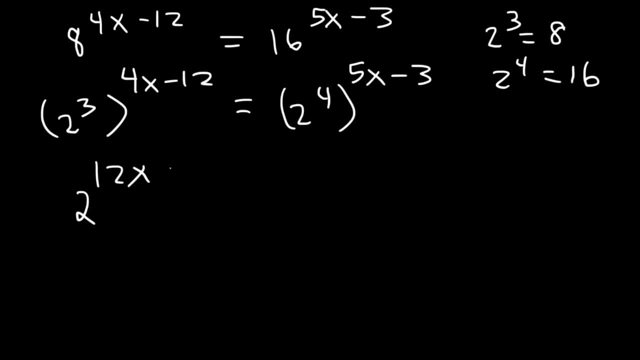 4x times 3 is 12x. 3 times negative. 12 is negative 36.. Now we need to multiply 5x minus 3 by 4. So that's going to give us 20x minus 12.. 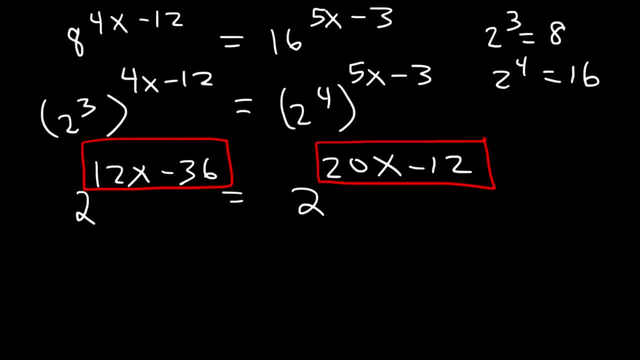 So we can set these two equal to each other Now that we have the same base. So 12x minus 36 is equal to 20x minus 12.. Let's subtract both sides by 12x. Let's add 12 to both sides. 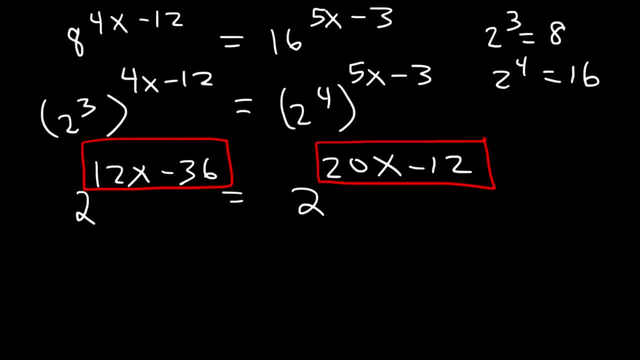 So we can set these two equal to each other Now that we have the same base. So 12x minus 36 is equal to 20x minus 12.. Let's subtract both sides by 12x. Let's add 12 to both sides. 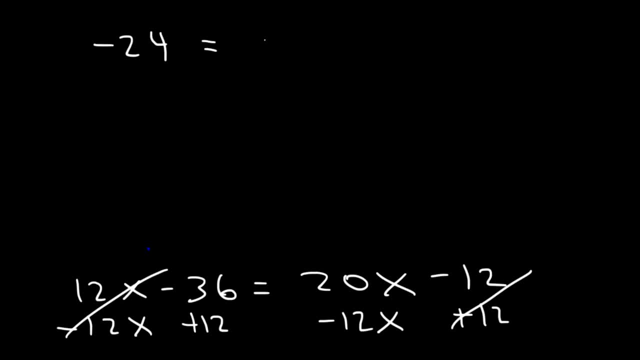 So negative 24. Is equal to 8x. Therefore x is equal to negative 3.. Let's try one more example: 27 raised to the 3x minus 2.. Let's say that's equal to 81 raised to the 2x plus 7.. 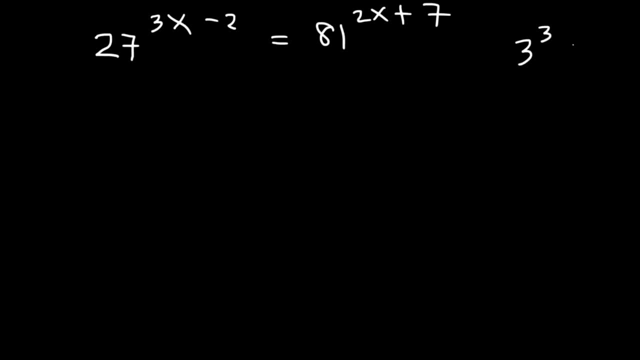 So try this problem Now: 3 to the third power is equal to 27.. And 3 to the fourth power is equal to 81. So let's replace 27 with 3 cubed And let's replace 81 with 3 to the fourth power. 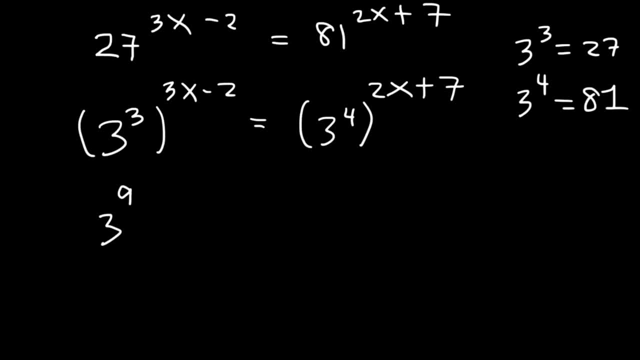 3 times 3x minus 2.. That's going to be 9x minus 6.. And 4 times 2x plus 7. That's 8x plus 28.. So now that we have the same base, we can set the exponents. 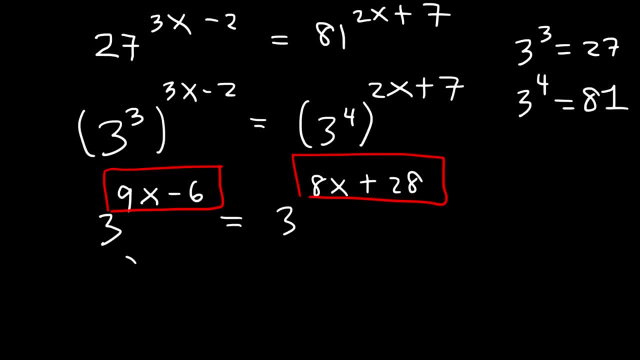 Exponents equal to each other. So 9x minus 6 is equal to 8x plus 28.. So let's subtract both sides by 8x And let's add 6 to both sides, So these will cancel. 9x minus 8x is x. 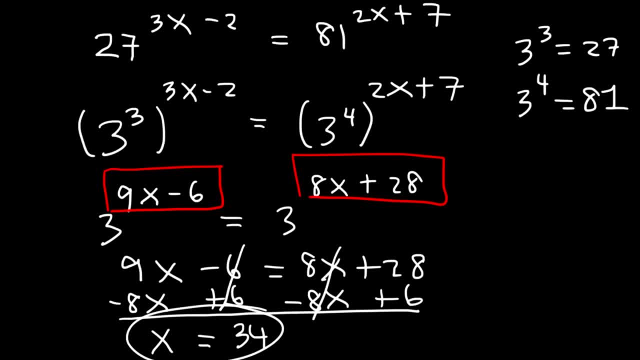 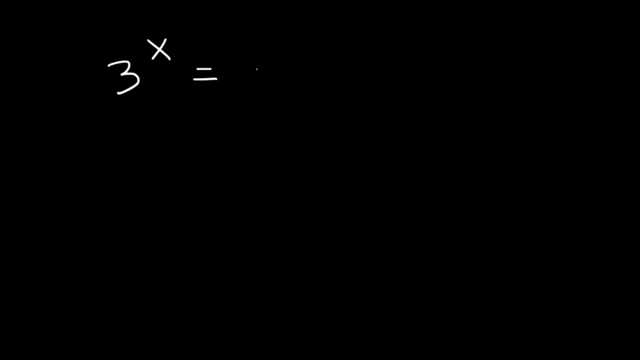 28 plus 6 is 34.. So x is equal to 34 in this example. Thank you, 3 raised to the x is equal to 8.. What is the value of x? In order to find it, we can take the log or the natural log of both sides. 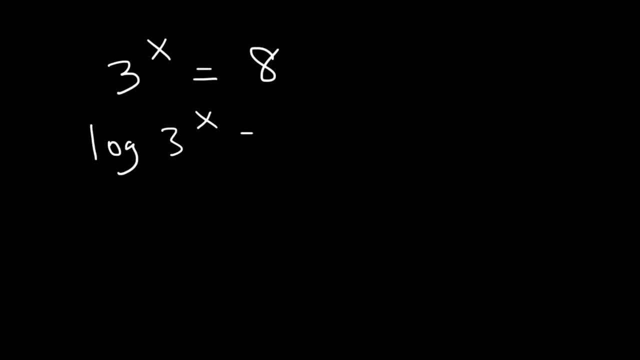 It really doesn't matter which one you're going to use. Let's take the log of both sides. Once you do that, you can move the exponent to the front. So x, log 3 is equal to log 8.. So x is log 8.. 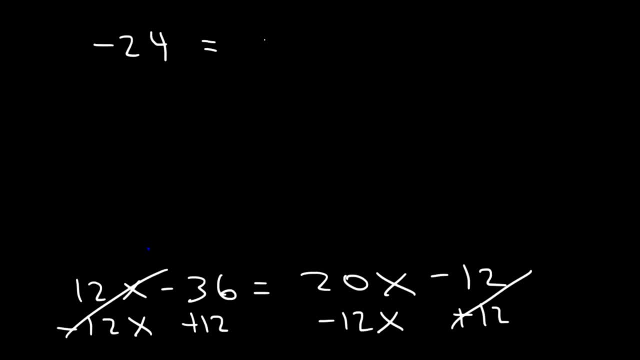 So negative 24. Is equal to 8x. Therefore x is equal to negative 3.. Let's try one more example: 27 raised to the 3x minus 2.. Let's say that's equal to 81 raised to the 2x plus 7.. 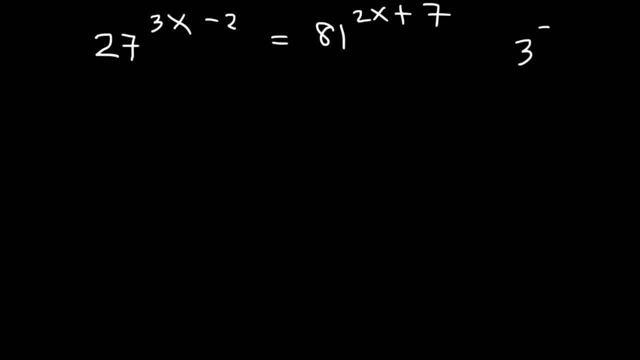 So try this problem Now: 3 to the third power is equal to 27.. And 3 to the fourth power is equal to 81. So let's replace 27 with 3 cubed And let's replace 81 with 3 to the fourth power. 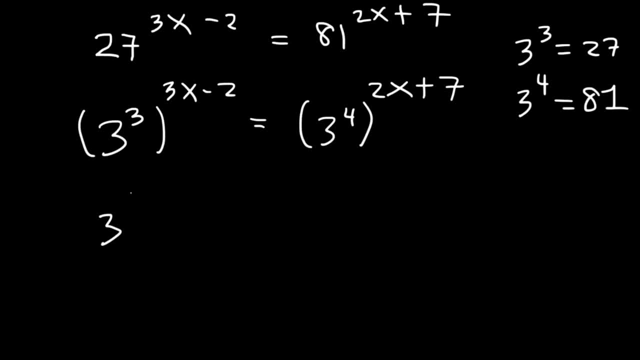 3 times 3x minus 2.. That's going to be 9x minus 6.. And 4 times 2x plus 7. That's 8x plus 28.. So now that we have the same base, 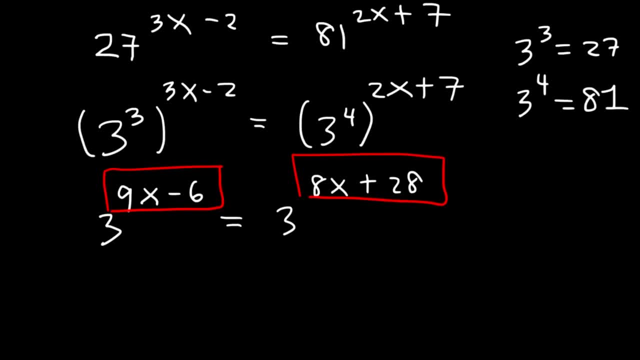 We can set the exponents Equal to each other. So 9x minus 6 is equal to 8x plus 28.. So let's subtract both sides by 8x And let's add 6 to both sides, So these will cancel. 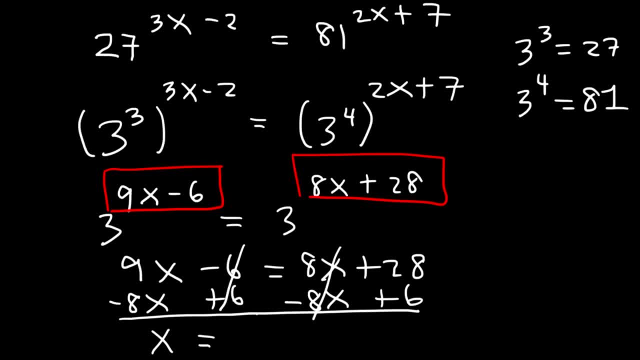 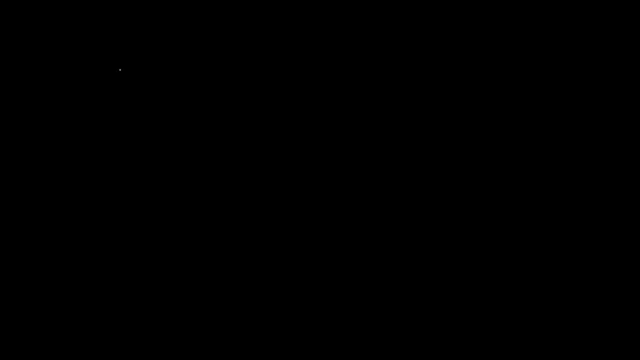 9x minus 8x is x, 28 plus 6 is 34.. So x is equal to 34. in this example, 3 raised to the 3x And it's not equal to 8x ल. Then the following one can be used as the punch line: 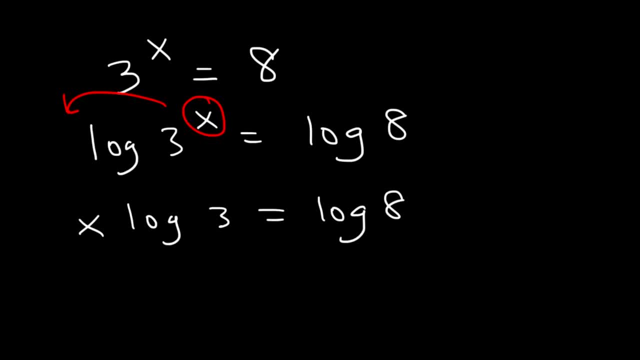 We can divide the force between good and bad, So it's going to be our periodic difference: Let's魚 divided by log 3.. If you type this in, you should get 1.8928.. And you can check your. 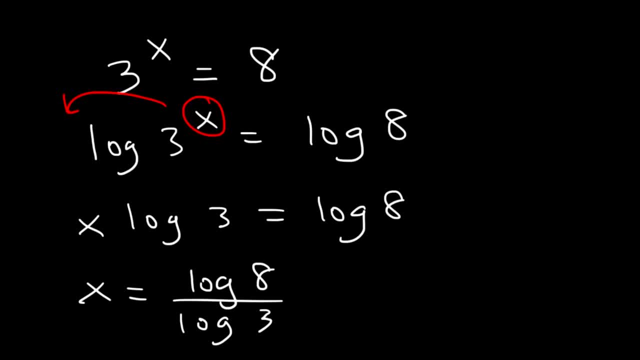 Divided by log 3.. If you type this in, you should get 1.8928.. And you can check your answer. What is 3 raised to the 1.8928?? If you type that in, the calculator will give you this answer. 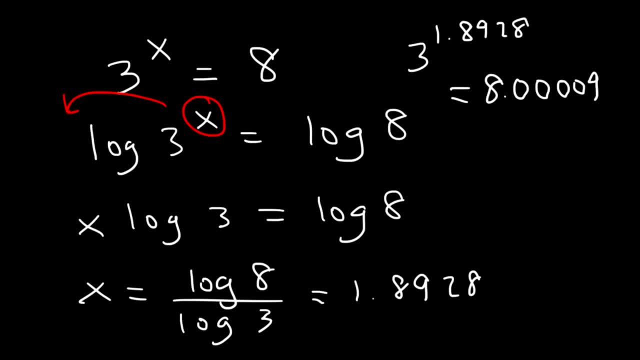 8.000.. 0.009.. Granted, this is rounded, so this is going to be very close to 8.. What about this one? If e raised to the x is equal to 7,, what is the value of x? 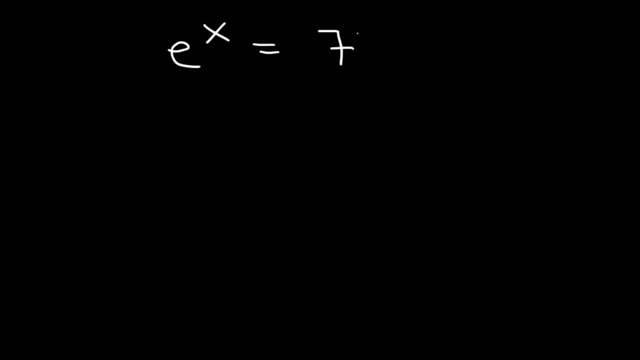 Now, whenever you're dealing with base e, it's better to use the natural log as opposed to the regular log. So we're going to take the natural log of both sides And we're going to move x To the front. So x ln e is equal to ln 7.. 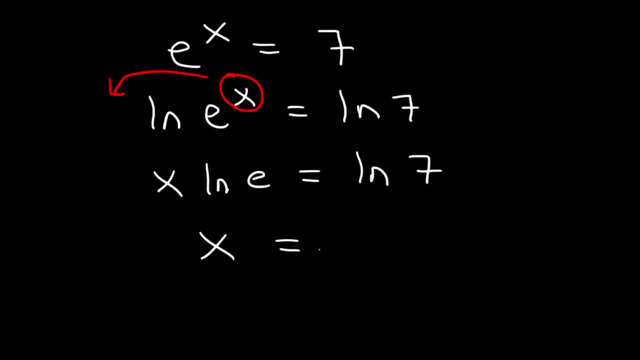 And ln e is 1.. So x times 1 is x. So the answer is ln 7.. This is the exact answer, And then you can type it in if you want the decimal answer. So the decimal answer is 1.9459.. 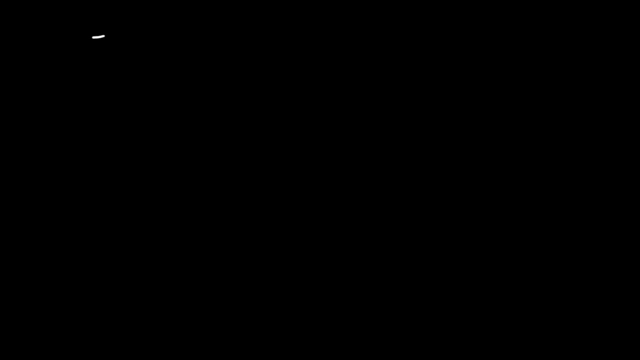 So that's the approximation. Now let's work on this example: 5 plus 4, raised to the x minus 2, is equal to 23. Let's find the value of x. So let's begin by subtracting both sides by 5. We can't take the log of both sides yet. 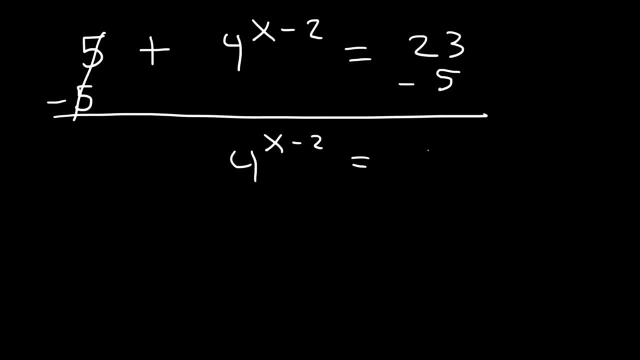 It wouldn't be wise. 23 minus 5 is 18. Now at this point we can't really convert 18 into a base 2. 2 to the 4th is 16,, 2 to the 5th is 32, So we can't really change 18 to a base 2. 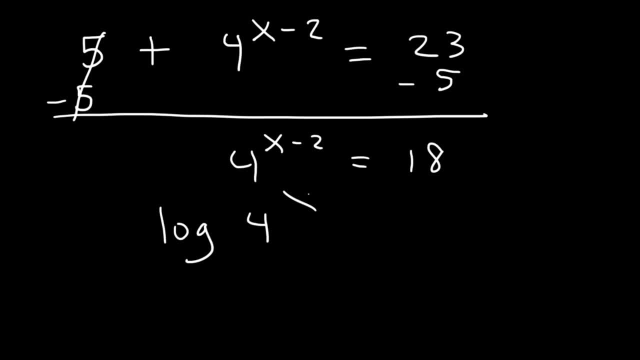 So we have to take the log of both sides. You can also use the natural log too. It will work as well. Now we can move the exponent to the front, And so it's x minus 2 in parentheses times, log 4, So we can move the exponent to the front. 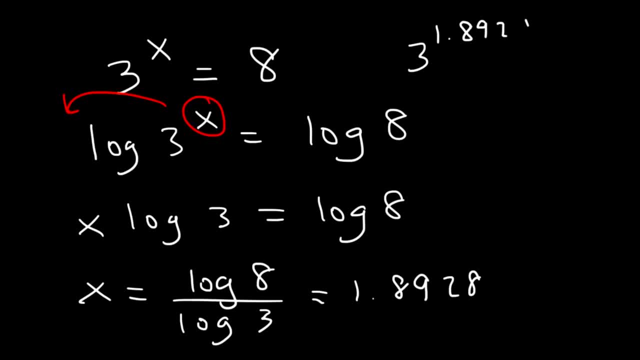 answer: What is 3 raised to the 1.8928?? If you type that in, the calculator will give you this answer: 8.00009.. Granted, this is rounded, so this is going to be very close to 8.. What about this one? If e raised to the x is equal to 7,, what is the value of? 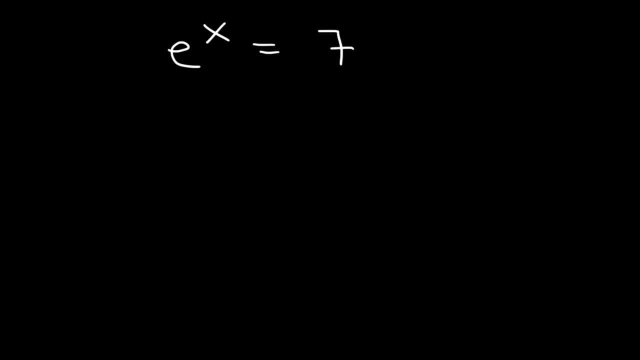 x. Now, whenever you're dealing with base e, it's better to use the natural log as opposed to the regular log. So we're going to take the natural log of both sides And we're going to move x to the front. So x ln e is equal to ln 7. And ln e is 1,. 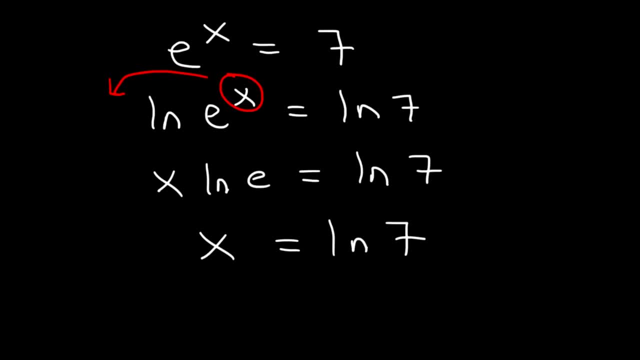 so x times 1 is x. So the answer is ln 7.. This is the exact answer And then you can type it in if you want the decimal answer. So the decimal answer is 1.9459.. So that's the answer, And then you can type it in if you want the decimal answer. So the decimal 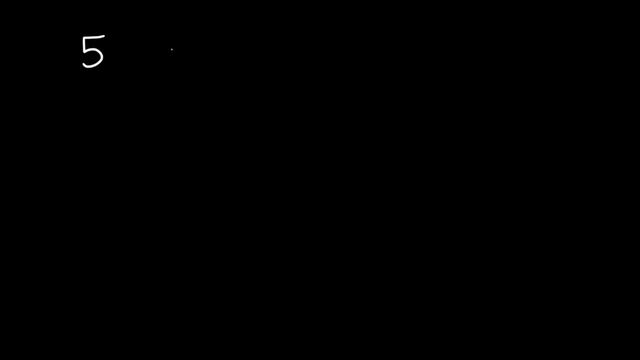 answer is 1.9459.. So the decimal answer is 1.9459.. So the decimal answer is 1.9459.. So that's the approximation. Now let's work on this example: 5 plus 4 raised to the x. 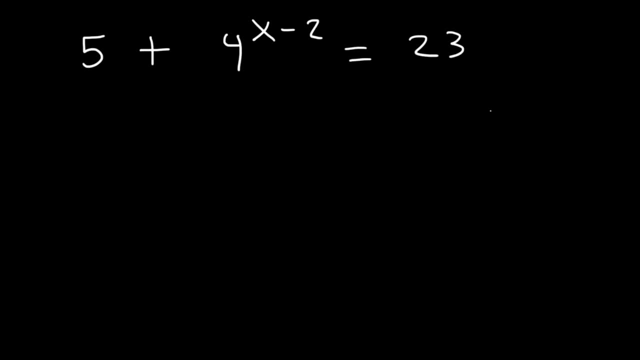 minus 2 is equal to 23.. Let's find the value of x. So let's begin by subtracting both sides by 5.. We can't take the log of both sides yet. It wouldn't be wise. 23 minus 5. 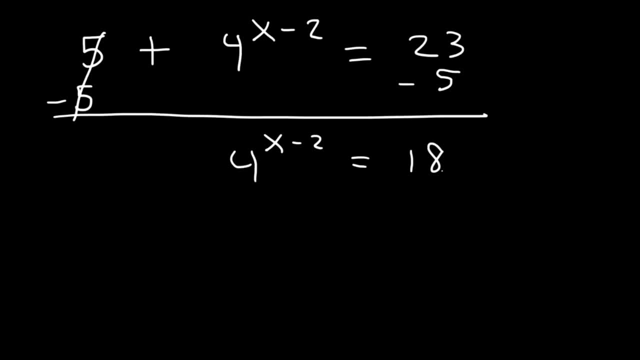 is 18.. Now, at this point we can't really convert 18 into a base: 2.. 2 to the 4th is 16.. 2 to the 4th is 16.. 2 to the 4th is 18.. 2 to the 4th is 16.. 2 to the 4th is: 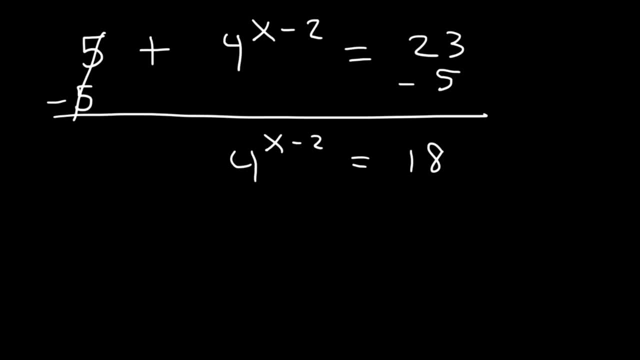 2 to the 5th is 32.. So we can't really change 18 to a base 2.. So we have to take the log of both sides. You can also use the natural log 2.. It will work as well. Now we can move. 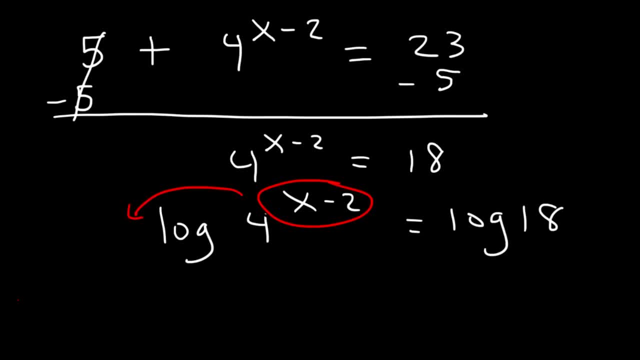 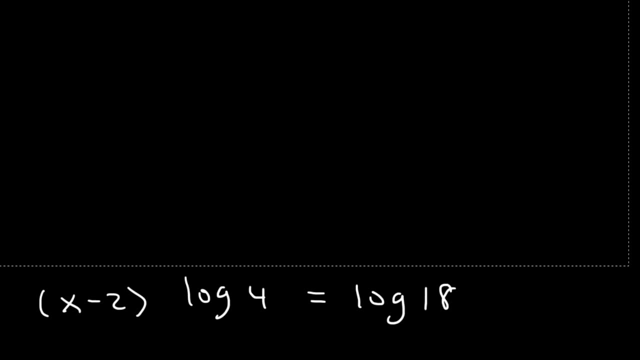 the exponent to the front, And so it's x minus 2, in parentheses times log 4. And that's equal to log 18.. I wouldn't recommend distributing log 4 to x minus 2.. Instead, it's better to divide both. 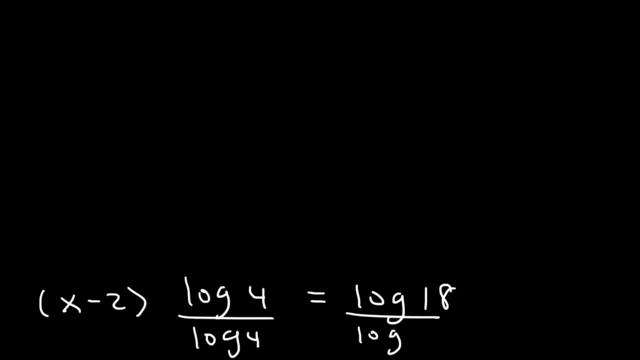 sides by log 4.. So x minus 2 is equal to log 18.. Well, let's get the exact answer first. So this is equal to log 18 over log 4.. The exact answer is this: x is equal to 2. 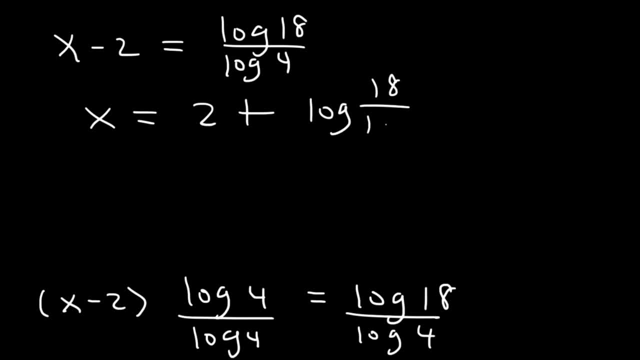 plus log 18 over log 4.. Log 18 divided by log 4, that's about 2.08496. And if we add 2 to it we can see that x is equal to 4.08496.. So that's the answer. Let's try this problem: 3 plus 2e raised to the 3 minus x. let's say: 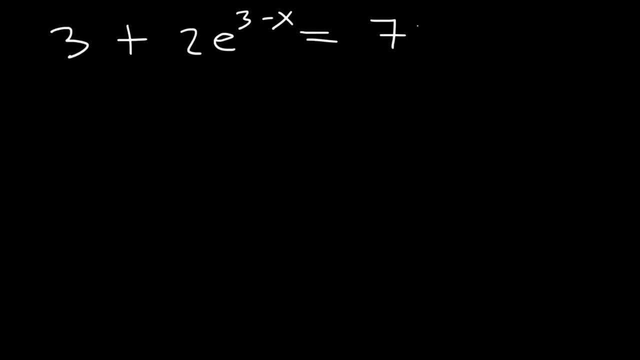 it's equal to 7.. Go ahead and find the value of x. So before we take the natural log of both sides, let's subtract both sides by 3.. So 2e to the 3 minus x is equal to 4.. Next, 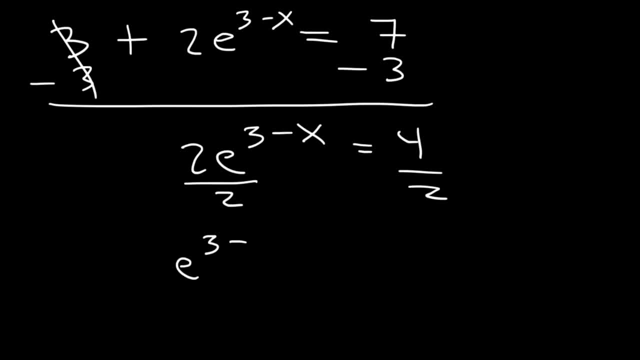 let's divide both sides by 2.. So e to the 3 minus x is equal to 2.. And now we can take the natural log of both sides. Now let's move the exponent to the front. So 3 minus x times ln e is equal to ln 2. And ln e is 1, so this is just going to be. 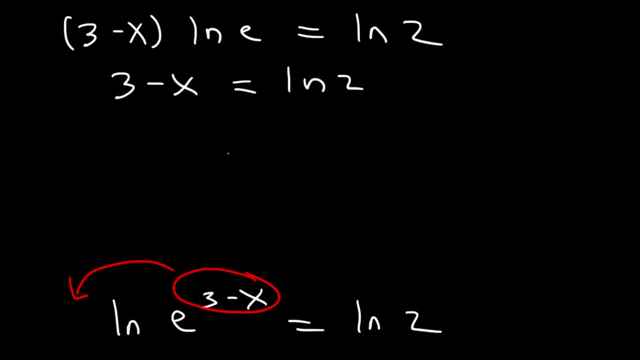 3 minus x. Now what I'm going to do is take the negative x and move it to this side. It's negative x on the left side, but it's going to be positive x on the right side. Now I'm. 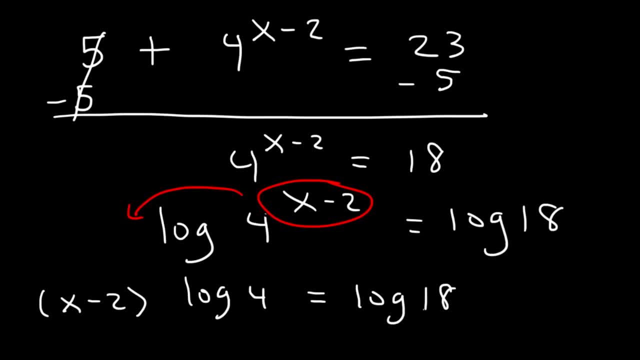 And so it's x minus 2, in parentheses, times log 4, And that's equal to log 18. I wouldn't recommend distributing log 4 to x minus 2. Instead, it's better to divide both sides by log 4, So x minus 2 is equal to log 18. 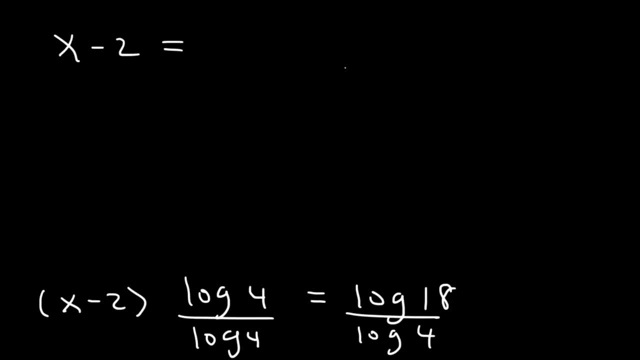 Well, let's get the exact answer first. So this is equal to log 18 over log 4. The exact answer is log 18 over log 4. The answer is this: x is equal to 2 plus log 18 over log 4. Log 18 divided by log 4. 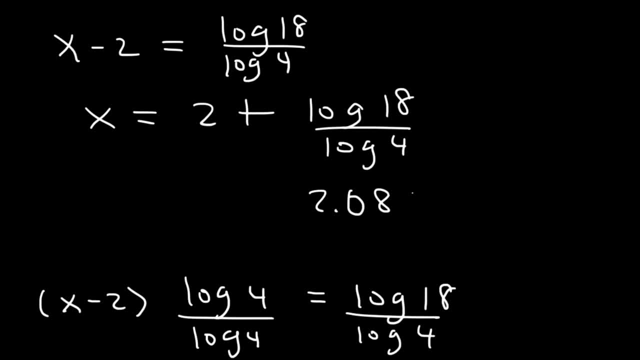 That's about 2.08496, And if we add 2 to it We can see that x is equal to 4.08496. So that's the answer. Let's try this problem: 3 plus 2, e raised to the 3 minus x. 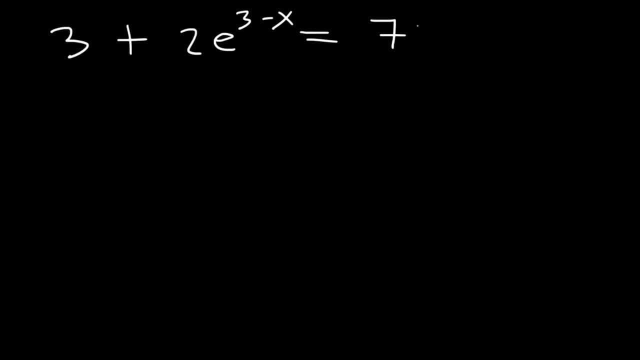 Let's say it's equal to 7. Go ahead and find the value of x. So before we take the natural log of both sides, Let's subtract both sides by 3, So 2 e to the 3 minus x is equal to 4. Next let's divide by 3. 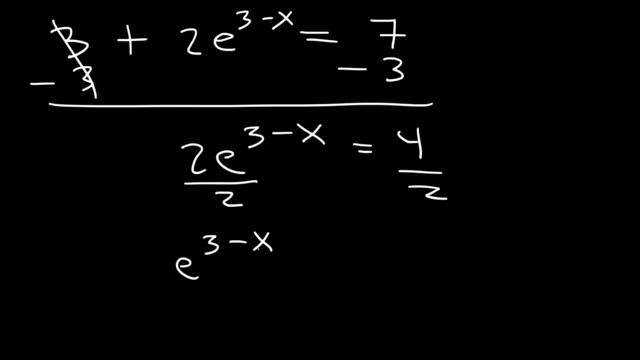 And we can also subtract both sides by 2. So e to the 3 minus x is equal to 2. And now we can take the natural log of both sides. Now let's move the exponent to the front. So 3 minus x times ln e is equal to ln 2. 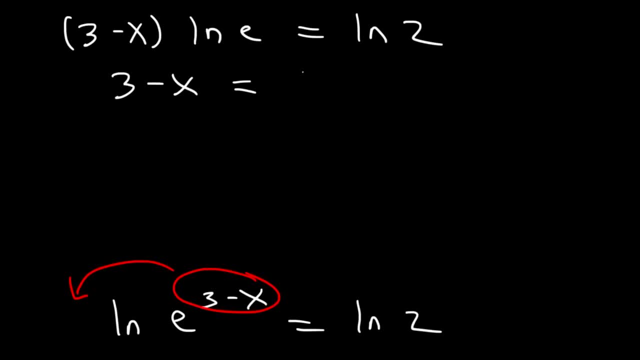 And L and E is 1, so this is just going to be 3 minus X. Now what I'm going to do is take the negative X and move it to this side. It's negative X on the left side, but it's going to be positive X on the right side. 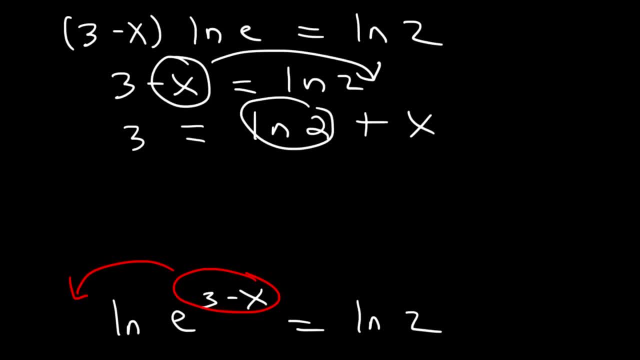 Now I'm going to take L and 2 and move it to this side, which is going to change from positive to negative. So X is 3 minus L and 2.. That's the exact answer. The decimal value is 2.3069.. 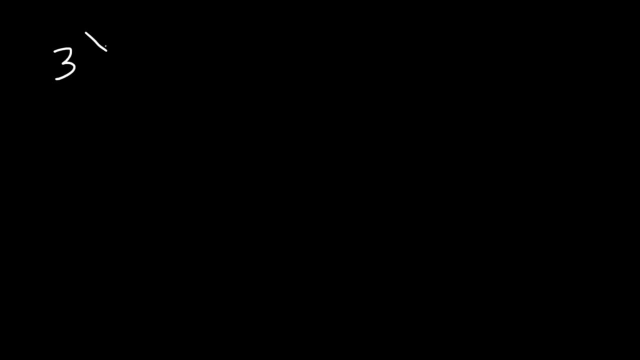 How would you solve this equation, 3 raised to the X squared plus 4.. Let's say that's equal to 1 over 27.. What would you do in order to find the value of X In this case? we know that. 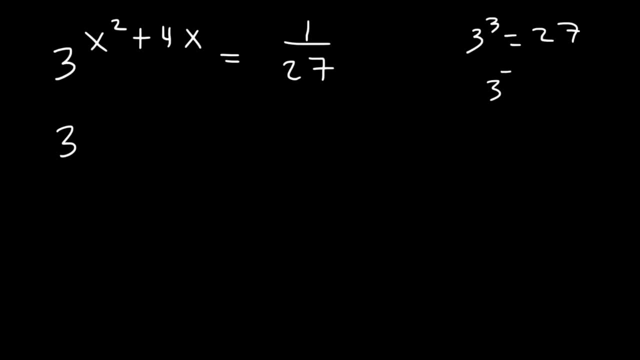 3 to the 3rd is equal to 27,. so 3 to the negative 3 is 1 over 27.. We need to make the bases the same, So this is 3 to the negative 3.. Because the bases are the same, we can now make the exponents equal to each other. 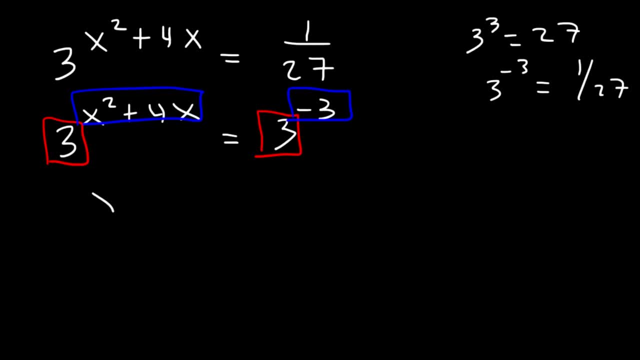 which means that X squared plus 4X is equal to negative 3.. Now let's move the negative 3 to the left side, In which case it's going to be positive 3, and we can factor Two numbers that multiply to 3 but add to 4 are 3 and 1.. 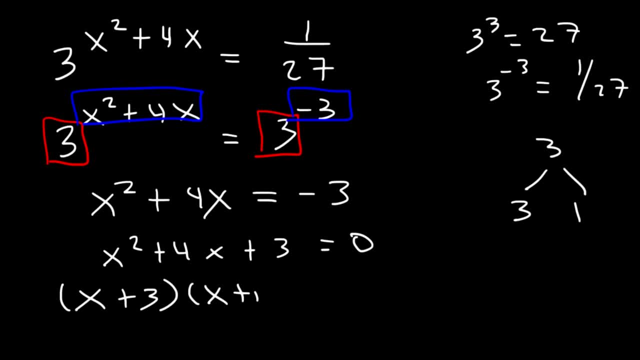 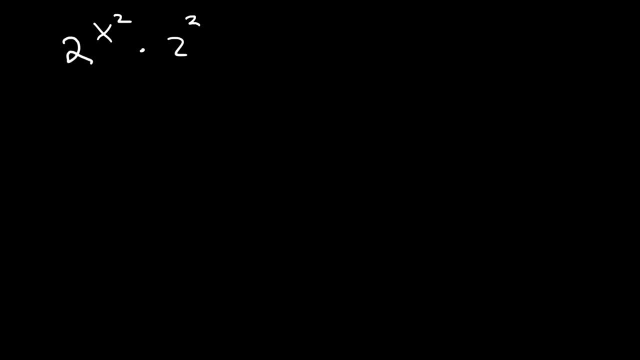 So this is X plus 3 and X plus 1.. So, therefore, X can be equal to negative 3 and X is equal to negative 1.. Here's another example: 2 raised to the X, squared times 2 raised to the 3X, is equal to 16.. 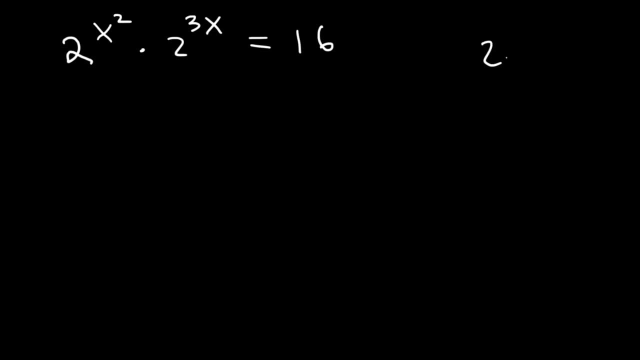 Find the value of X, 2 to the 4th is equal to 16, so let's replace 16 with that. Now let's say: if you're multiplying by a common base, You can add the exponents: 2 plus 3 is 5.. 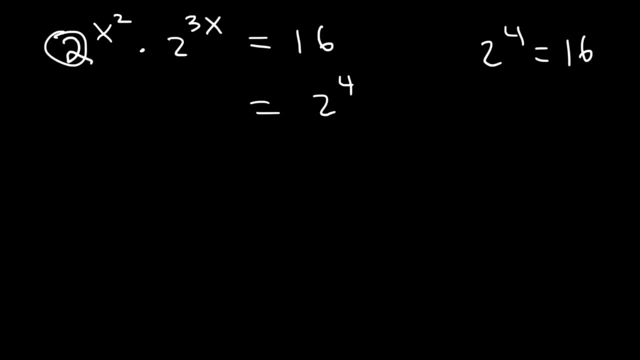 In this case, 2 is the common base, So we can add X squared and 3X. So this is 2X squared plus 3X. So now we can set X squared plus 3X equal to 4.. 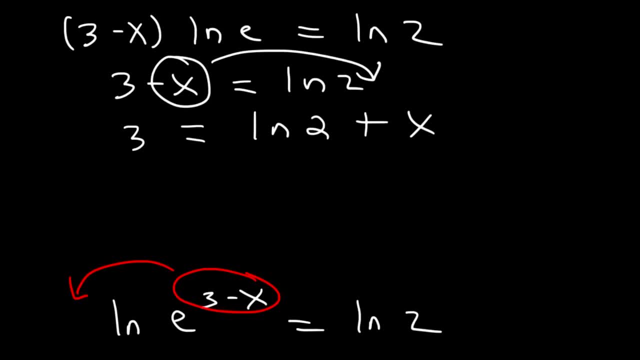 going to take ln 2 and move it to this side, which is going to change from positive to negative. So x is 3 minus ln 2.. That's the exact answer. The decimal value is 2.3069.. How would you solve this equation? 3 raised to the x squared plus 4.. Let's say: 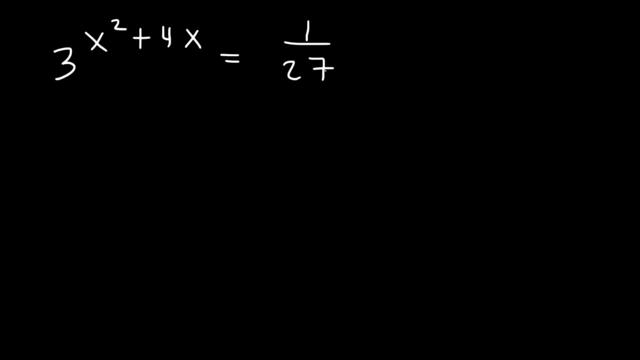 that's equal to 1 over 3.. What would you do in order to find the value of x In this case? we know that 3 to the third is equal to 27.. So 3 to the negative 3 is 1 over 27.. We need to make the bases. 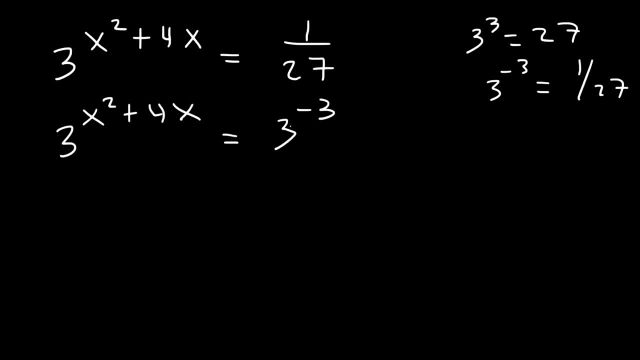 the same. So this is 3 to the negative 3.. Because the bases are the same, we can now make the exponents equal to each other, which means that x squared plus 4x is equal to 1 over 27.. 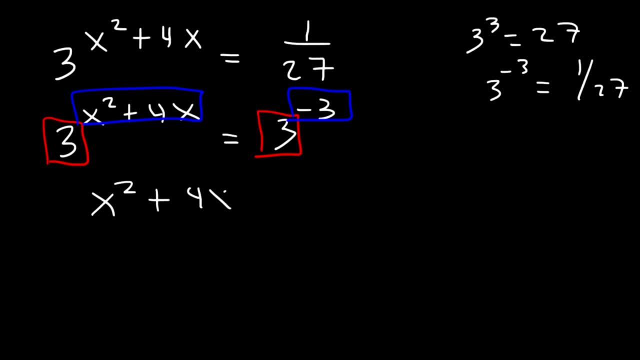 2 to the negative 3 is equal to negative 3.. Now let's move the negative 3 to the left side, which in this case is going to be positive 3, and we can factor Two numbers that multiply to 3 but add to 4 are 3 and 1.. So this is x plus 3 and x plus 1.. So therefore, x can: 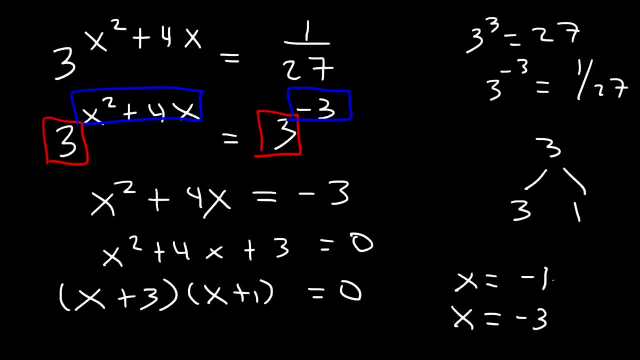 be equal to negative 3 and x is equal to negative 1.. Here's another example: 2 raised to the x squared plus 2 is 2 over 27.. var x squared plus 1 is 1 over 27.. Here's another example. 2 raised to the x squared plus 2 x squared is 1 over 27.. So x is equal to negative 1. It's simple economy: log x. but it's not the answer to this. That's because your value is 2 over 29.. 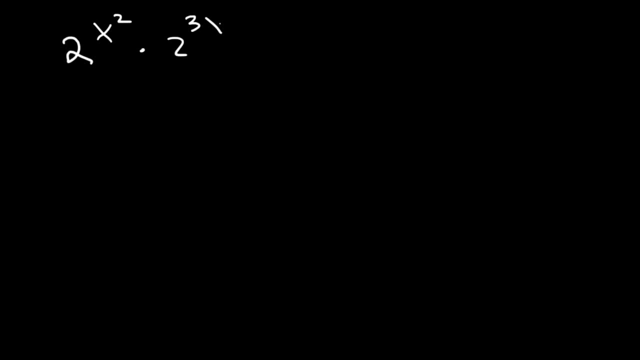 to the x, squared times 2, raised to the 3x, is equal to 16.. Find: the value of x, 2 to the 4th is equal to 16, so let's replace 16 with that. Now let's say if you're multiplying by a common base: 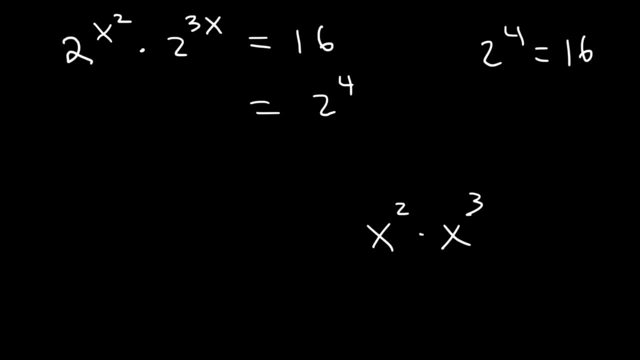 you can add the exponents: 2 plus 3 is 5.. In this case, 2 is the common base, so we can add x squared and 3x. So this is 2x squared plus 3x. 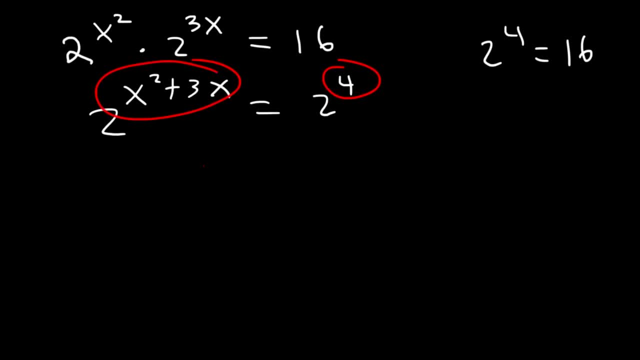 So now we can set x squared plus 3x equal to 4.. Now let's subtract both sides by 4.. So x squared plus 3x minus 4 is equal to 0, and let's factor Two numbers that multiply to negative 4,. 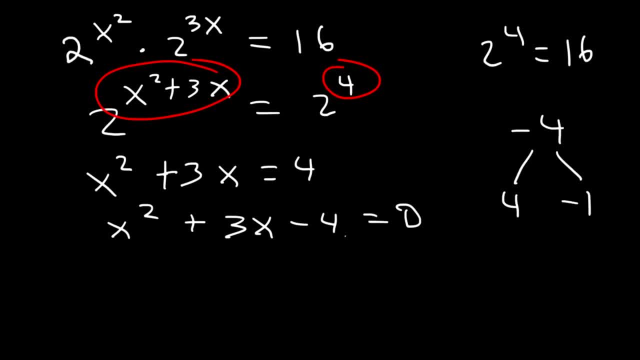 but add to positive 3, are positive 4 and negative 1.. So it's x plus 4 times x minus 1, which means that x is equal to negative 4 and it's equal to positive 1.. Try this: 4 raised to the 2x minus 20, multiplied by 4 raised to the x. 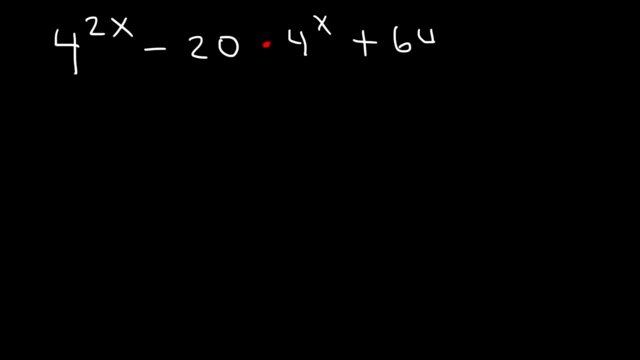 plus 16.. See x squared is equal to 0.. So what can we do in order to find the value of x? What I think we should do is factor, but factor by substitution. This equation can be reduced to a quadratic equation. 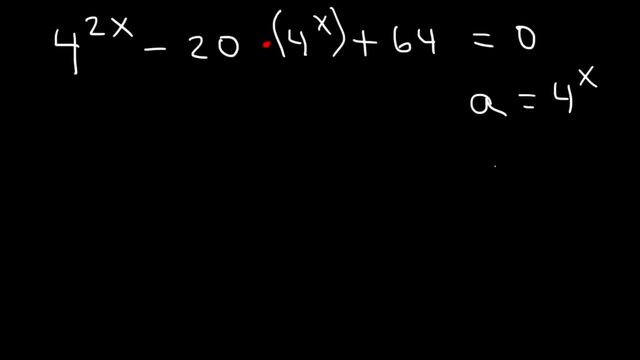 We're going to set a equal to 4 raised to the x, which means that a squared is 4 to the 2x. So let's set a equal to 4 raised to the x. Let's replace 4 to the 2x with a squared and let's replace 4 to the x with a. 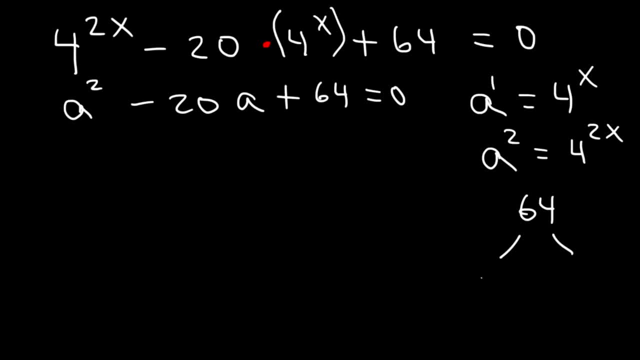 What two numbers multiply to 64 but add to negative 20? This is negative 16 and negative 4.. So to factor it, it's a minus 16 and a minus 4.. So therefore, a is equal to 16 and a is equal to 4.. 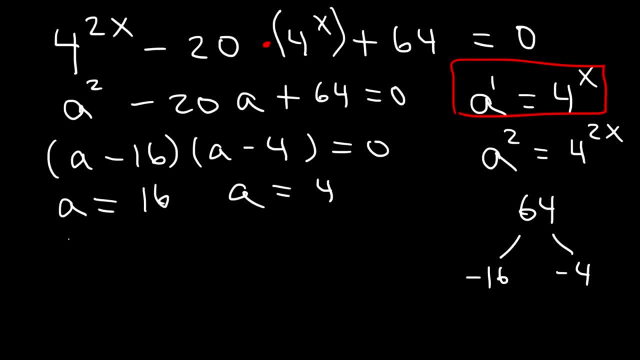 And we know that a is 4 to the x. So therefore, 4 raised to the x is equal to 16 and 4 to the x is equal to 4.. 4 is basically 4 to the first power, So we can clearly see that x is equal to 1.. 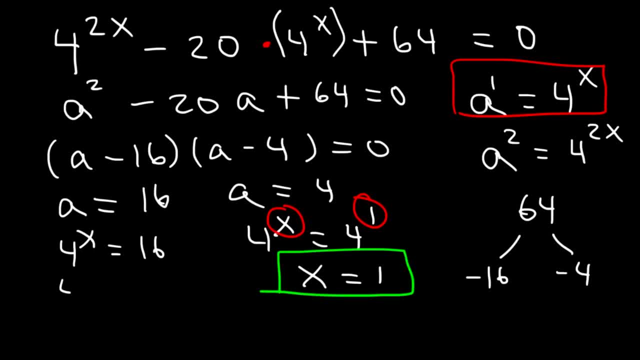 Now, 16 is equivalent to 4 squared. So 4 to the x is equal to 4 squared, which means that x is equal to 2.. And so those are the two answers. Let's try one more example: 3 to the 2x. 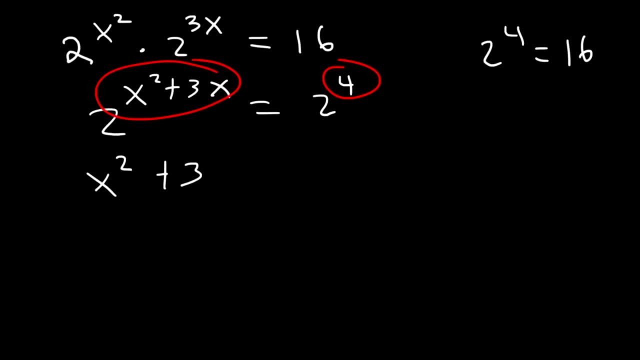 Now let's subtract both sides by 4.. So X squared plus 3X minus 4 is equal to 0.. Now let's factor Two numbers that multiply to negative 4 but add to positive. 3 are positive 4 and negative. 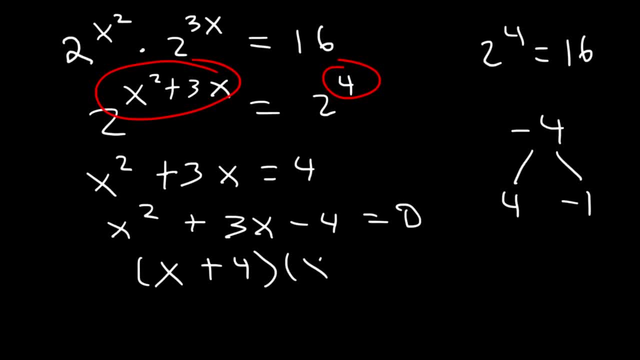 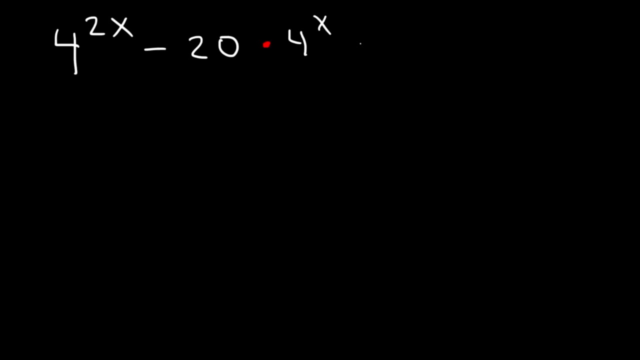 1. So it's X plus 4 times X minus 1, which means that X is equal to negative 4 and it's equal to positive 1.. Try this: 4 raised to the 2X minus 20, multiplied by 4 raised to the X plus 64, is equal to 0.. 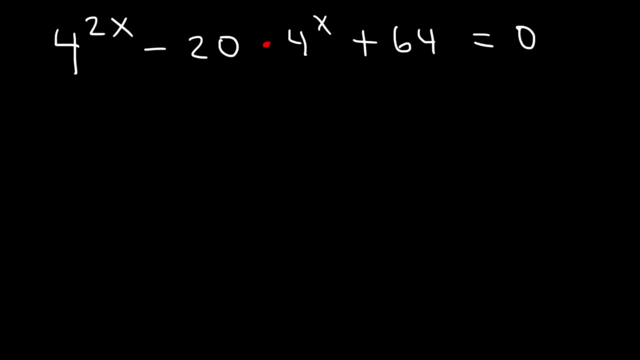 So what can we do in order to find the value of X? What I think we should do is factor, But factor by substitution. This equation can be reduced to a quadratic equation. We're going to set A equal to 4 raised to the X, which means that A squared is 4 to 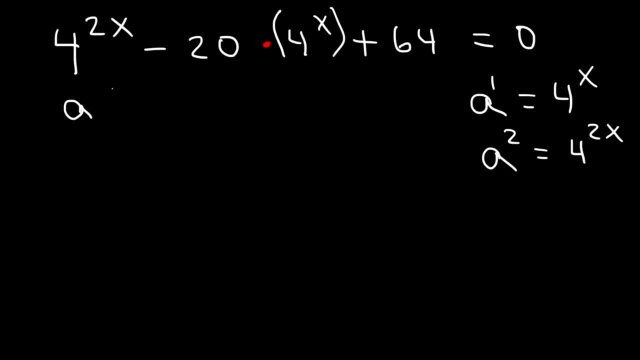 the 2X. So let's replace 4 to the 2X with A squared and let's replace 4 to the X with A. What two numbers multiply to 64 but add to negative 20? This is negative 16 and negative 4.. 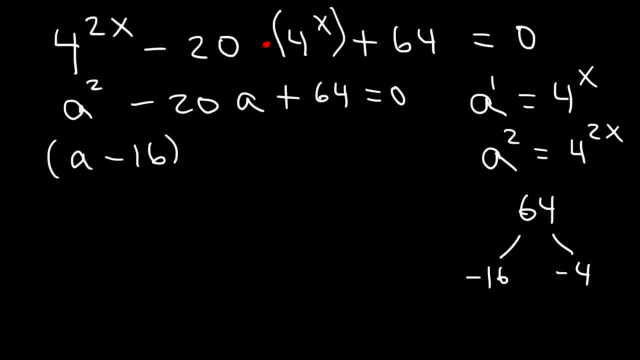 So, to factor it, it's A minus 16 and A minus 4.. So therefore, A is equal to 16 and A is equal to 4.. And we know that A is 4 to the X. So therefore, 4 raised to the X is equal to 16 and 4 to the X is equal to 4.. 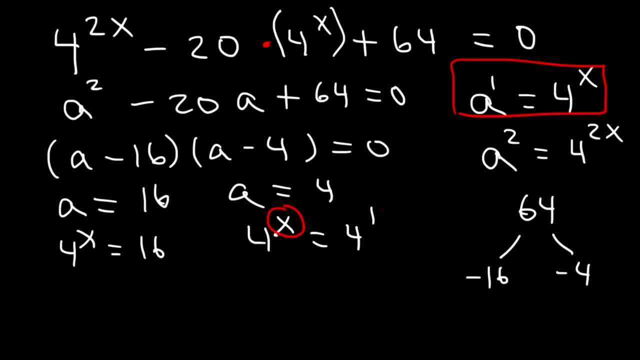 4 is basically 4 to the first power, So we can clearly see that X is equal to 1.. Now, 16 is equivalent to 4 squared, So 4 to the X is equal to 4 squared, which means that X is equal to 2.. 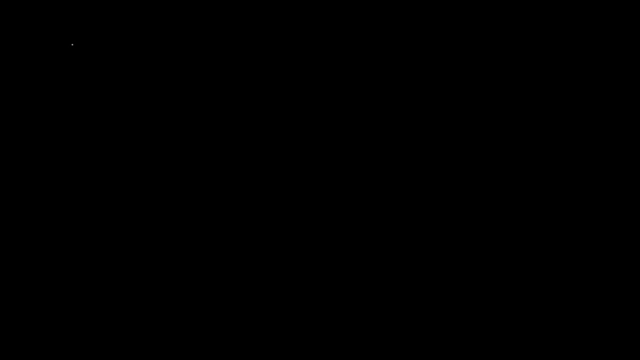 And so those are the two answers. Let's try one more example: 3 to the 2X minus 3 to the 2X minus 1.. Let's say it's equal to 18.. Go ahead and find the value of X. 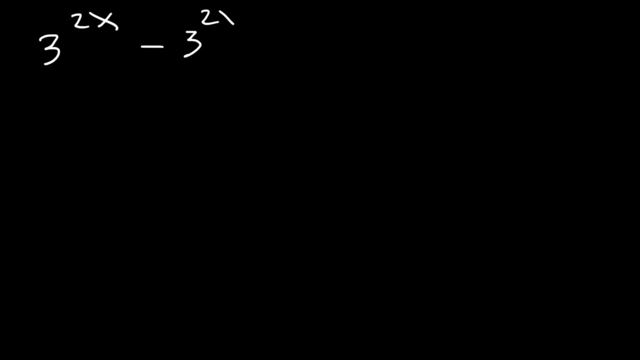 2x minus 3 to the 2x minus 1.. Let's say it's equal to 18.. Go ahead and find the value of x. So we can't really factor in this example, because 2x is not twice the value of 2x minus. 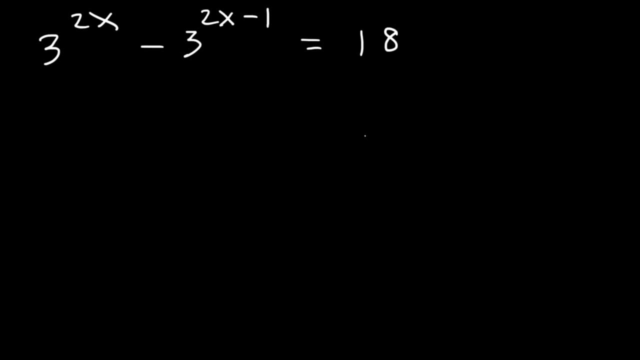 1. But we could factor the GCF. We could take out 3 to the 2x. 3 to the 2x divided by itself is equal to 4.. 3 to the 2x divided by itself is equal to 4.. 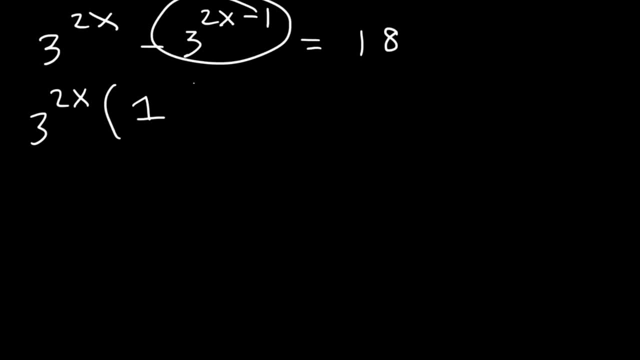 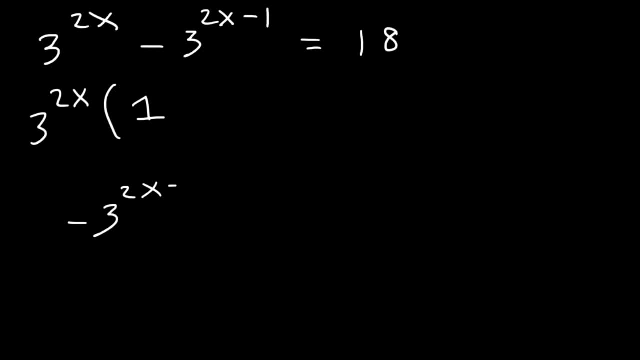 If we write it out, notice what we'll get. Let's ignore the negative sign for now We know the overall answer is going to be negative. When you divide by a common base, you need to subtract the exponents 2x minus 1 minus 2x. 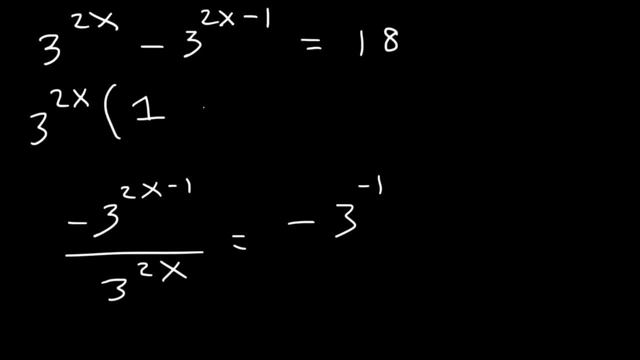 The 2x will cancel, And so it's going to be 3 to the negative 1.. And so it's going to be 3 to the negative 1.. So now we know the answer, and so that's what we have right now, And if you distribute, you can see that you're going to get. 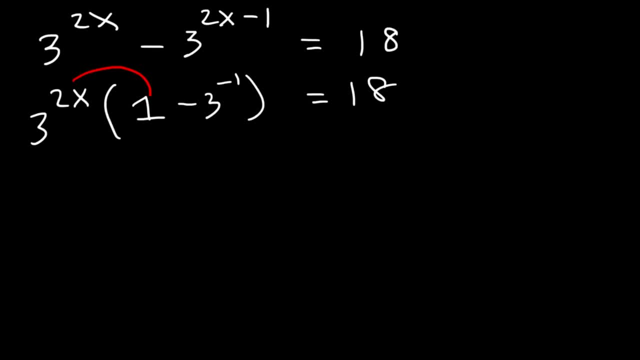 the original equation 3 to the 2x times 1 gives you this term, and 3 to the 2x times 3 to negative 1, you add the exponents 2x plus negative 1 is 2x minus 1.. Now let's divide both sides by this. 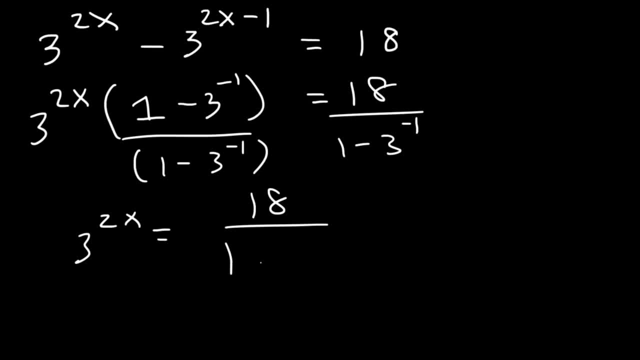 3 to the negative. 1 is basically 1- third. So we have a complex fraction. Let's multiply the top and the bottom by 3.. So 18 times 3 is 54.. 3 times 1 is 3.. 3 times 1: third is 1.. And 3 minus 1 is 2.. 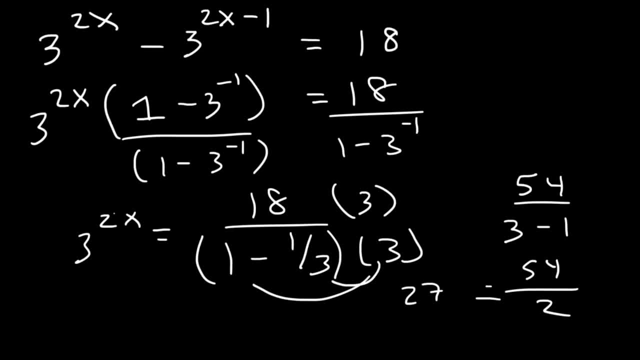 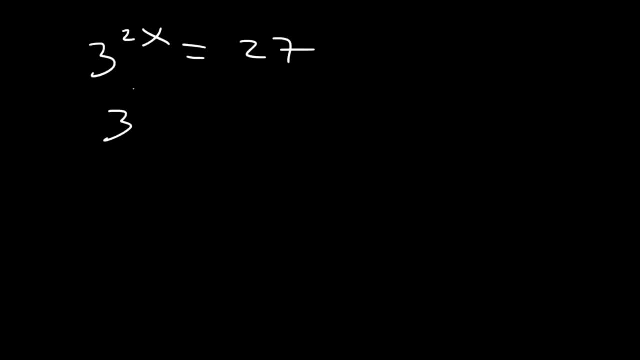 54 over 2 is 27.. So 3 to the 2x is equal to 27.. And 27 is 3 to the 3rd power. So 2x is equal to 3, which means that x is 3 over 2.. And so that's the answer. Thank you.